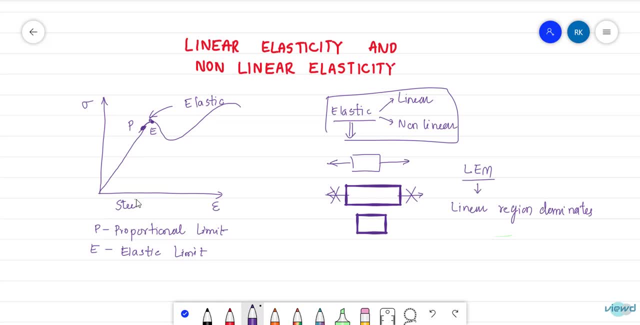 So, if you consider this, in the elastic region there is mostly linear nature. Consider this graph for steel: Up to here, up to this point E, the body is elastic, But up to proportional limit that is a straight line, It is a linear curve. So this can be called as linear elastic material. 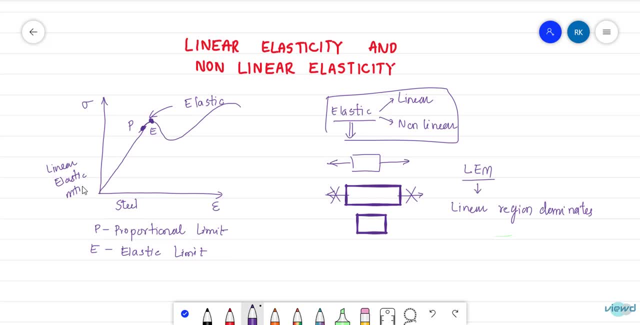 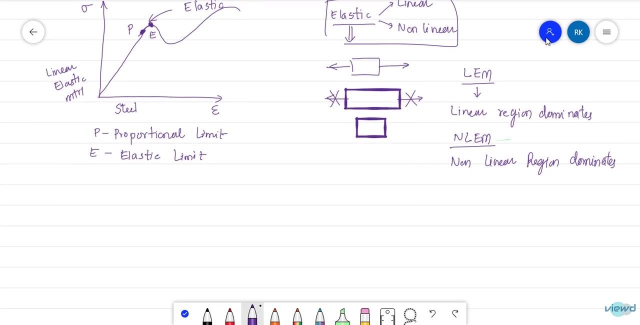 So what is non-linear elastic material? Non-linear elastic material, So non-linear region dominates. So in the elastic region if the curve is non-linear, or a non-linear region dominates, or linear region dominates, then it is non-linear, So this can be called as non-linear elastic material. 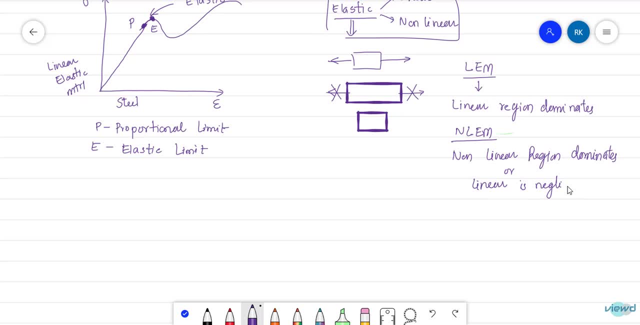 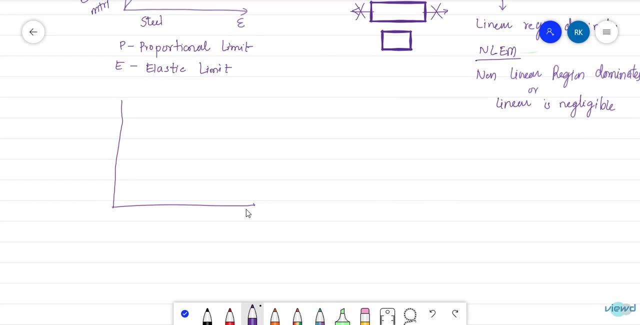 is negligible. this can be observed in case of rubber. so for rubber, stress strain graph will be theoretical. stress strain graph will be somewhat like this: this is during loading and during unloading the graph returns this way. so this is during unloading. so this is for rubber. if you see the graph, you can see. 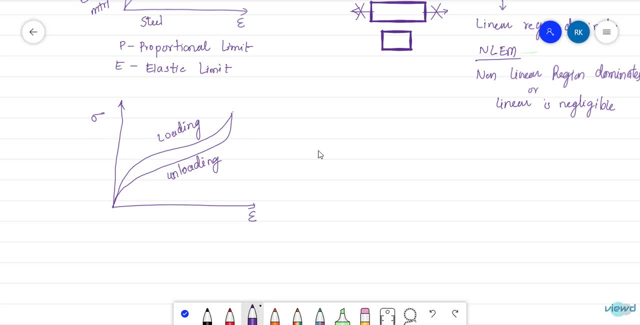 that there is no linear portion in the stress-strain graph, so this is nonlinear. nonlinear elastic material, nonlinear elastic. so this is the difference between elastic and nonlinear elastic material. then another misconception is that where to apply Hooke's law? so where to apply Hooke's law? 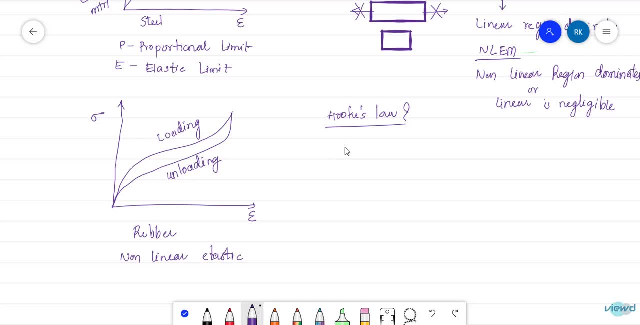 so first, what is Hooke's law? Hooke's law means see meeting at stress's directamente proportional to strain, and I think that is the thinner. so here is which is the linear one here: linear elastic material. you have to remove section here. there are three. 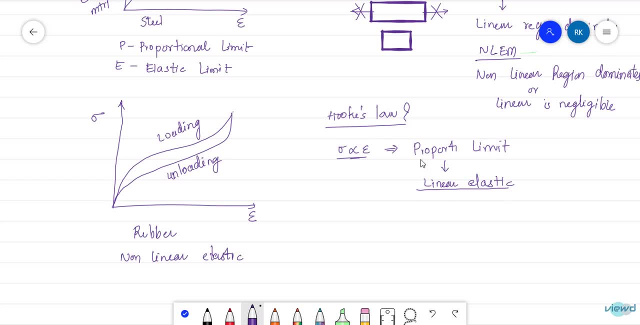 links. you will have single line each of these links, NHS main links. if we have a nonlinear elastic material that will serve linear elastic material, then H with you can be directly proportional to the stress and when you go to stress distribution it will melts with a straight line, so without distant stress. so this will be in proportional region up to proportional limit, up to proportional limit up to porte. 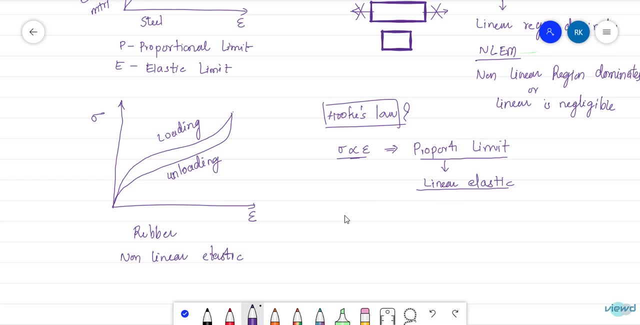 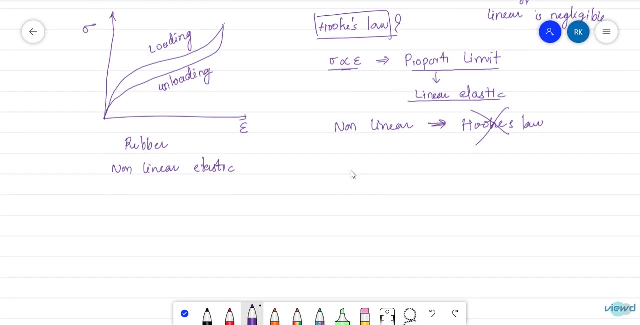 limit. we can apply this Hooke's law then for nonlinear elastic material. for nonlinear, we cannot apply Hooke's law. so we cannot apply Hooke's law for nonlinear material. and, as a confusion, is that Young's modulus. so what does this Young's modulus indicate? Young's modulus indicates how elastic, how much elastic. 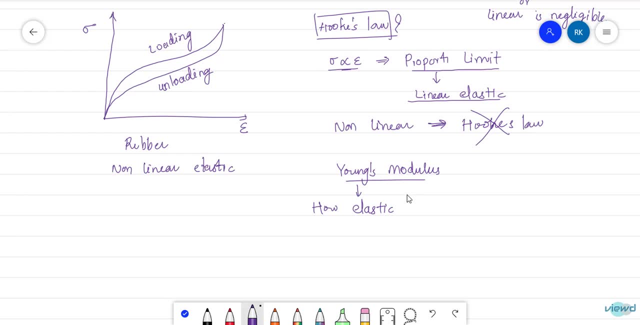 a material is. so Young's modulus can be easily understood by comparison. so now let us take steel and rubber. for steel this Young's modulus is some 2 into 10 power, 5 Newton per meter square, and for rubber is equal to some 1, 1 or 0.1 once check this. so for rubber it is. 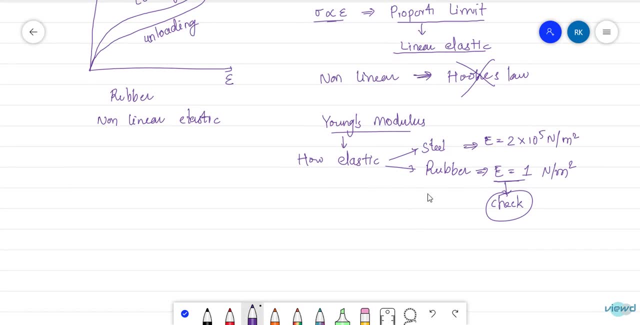 let us say 1 Newton per meter square. so for rubber this Young's modulus is very low. so by observing directly we can say that you can. you will say that the rubber is more elastic than steel, but it is wrong. so if elasticity is high, if Young's modulus is high, elasticity is low. if Young's 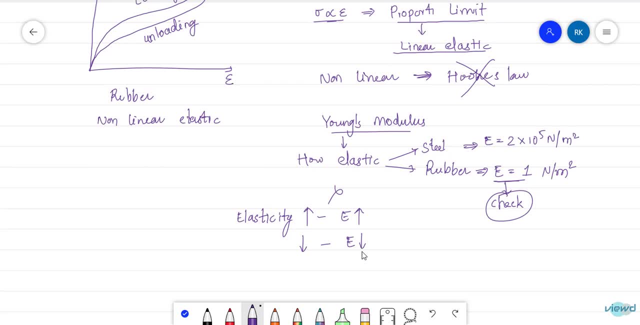 modulus is low. so what is this indicating is that you know that Sigma is directly proportional to strain, so Sigma is equal to E into epsilon and E is equal to Sigma by epsilon alone. so from this we can see that if there are two materials, steel and rubber, 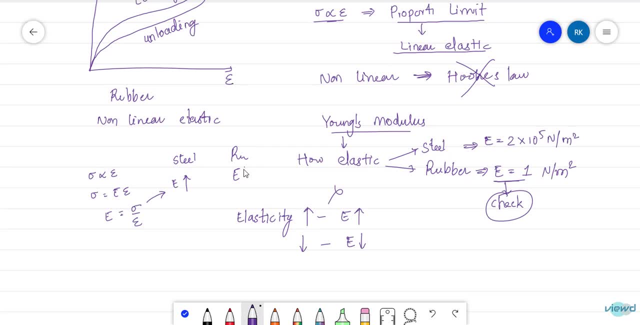 is high for steel is low for rubber. if E is high Sigma, this more stress is required to produce it, the permanent deformation. in case of rubber, less stress is required to produce permanent deformation. or we can say that if some hundred megapascal, hundred megapascal is applied in case of a steel, then it 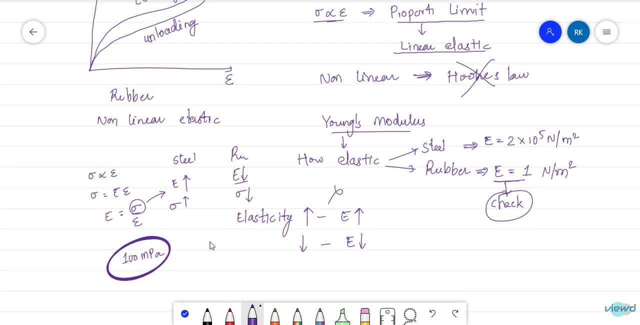 remains in the elastic region only. but in case of rubber, even if one Newton per mm square- sorry, greater than one Newton per meter square- is applied in case of rubber, then it goes beyond this elastic region. so that's what it is indicating. so you, even if we apply more stress in case of steel, that remains in the elastic. 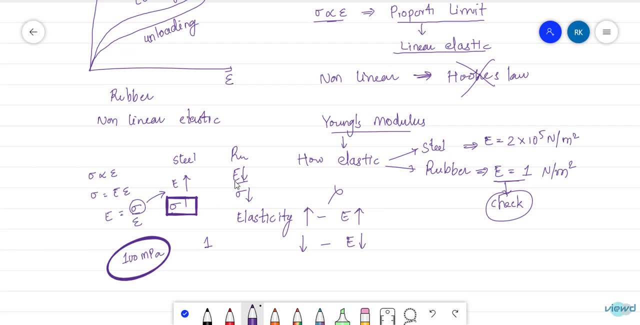 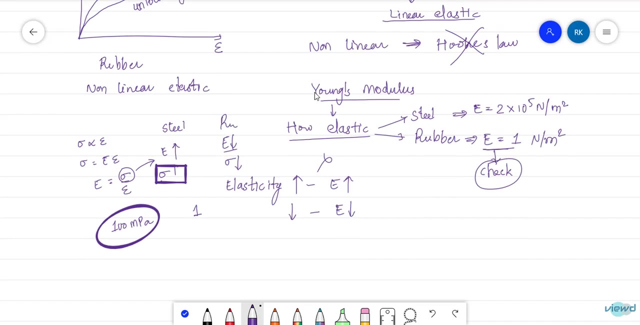 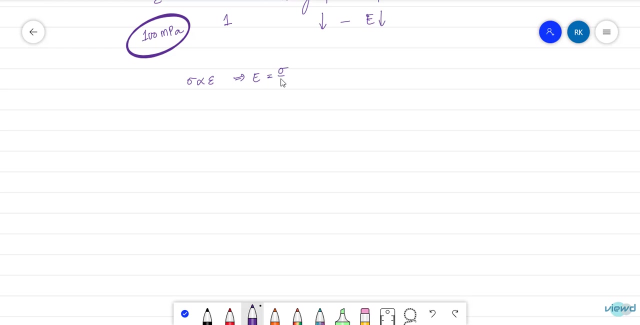 region, but in case of rubber it goes into the plastic region. so from this we can understand that Young's modulus indicates how elastic and how much strength does the material possess is represented with Young's modulus, and also Sigma is directly proportional to strain and from this we can get: E is equal to Sigma by 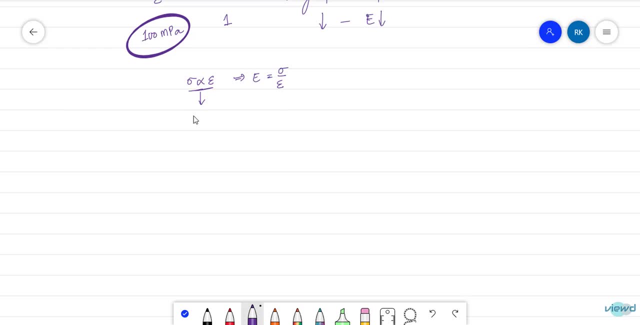 Epsilon. so Sigma is directly proportional to straightlan, where this is in up to proportional limit only. and this proportionality limit exists for linear elastic material. then what about this nonlinear elastic material? how to calculate this? Young's modulus for nonlinear elastic material? so, aah, young's modulus is generally constant for 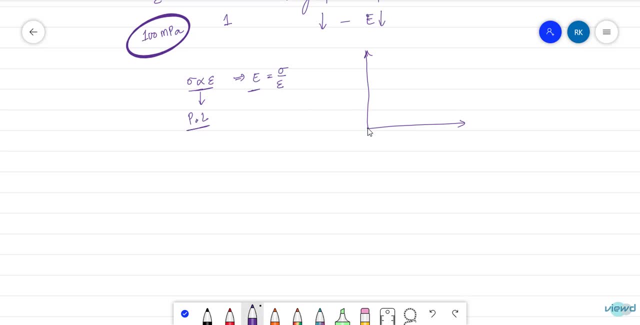 a single material. so if you consider the rubber, it, the graph will be like this. to strain graph will be like this, and for nonlinear materials, this Young's modulus can be calculated with average values up to considered stress level. so if you consider this point, the Young's modulus value will be slope at this point. if you